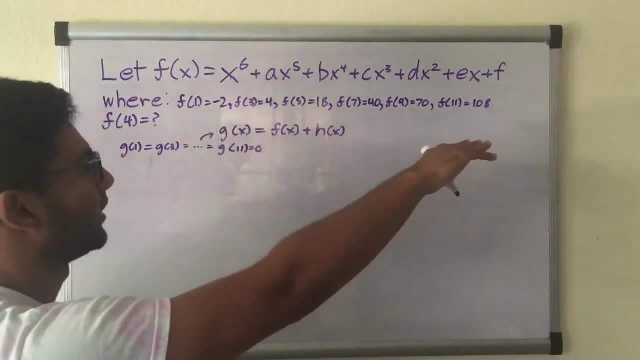 spit out an output equivalent to these outputs for f, and then we can subtract that, So actually I'll write f of x minus h of x, And then we can subtract that, So actually I'll write f of x minus h of x. 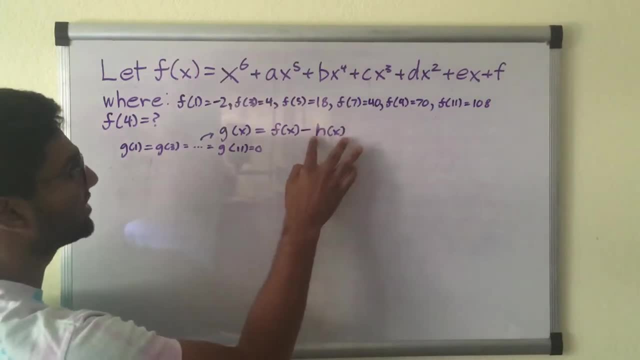 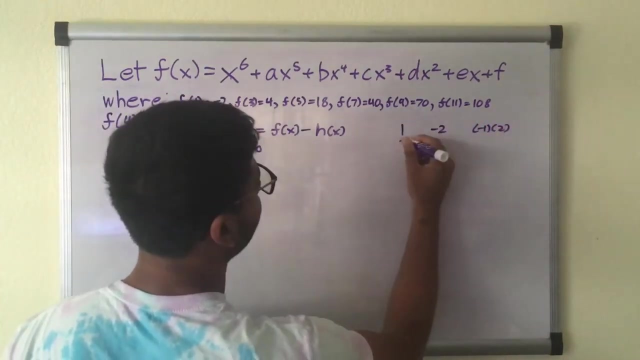 So that when we replace this h of x with a function we find, we will subtract the exact outputs that we get and we'll get zero for those initial values. So we do need to find a pattern first. So f of 1 is negative 2, this is negative 1 times 2.. f of 3 is 4, this is 1 times 4.. 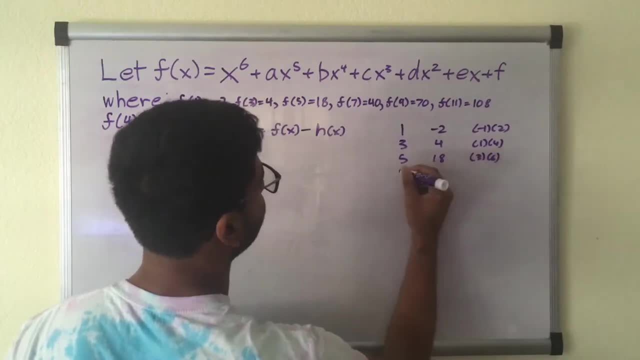 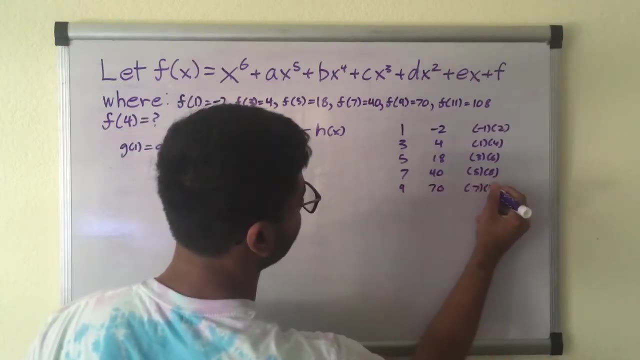 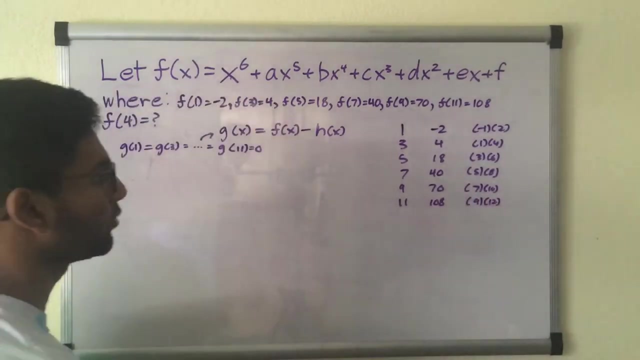 f of 5 is 18,, which is 3 times 6.. f of 7 is 40,, which is 5 times 8.. f of 9 is 70, or 7 times 10.. f of 11 is 108, which is 9 times 12.. So what we see here. 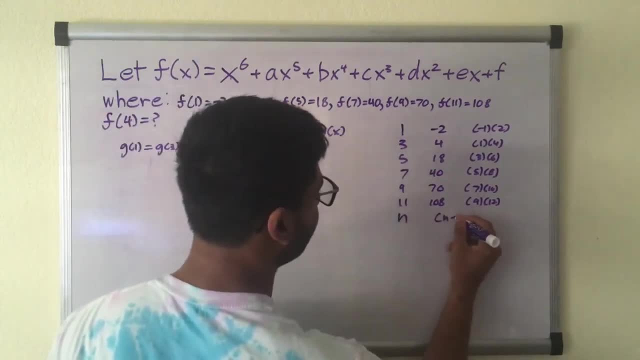 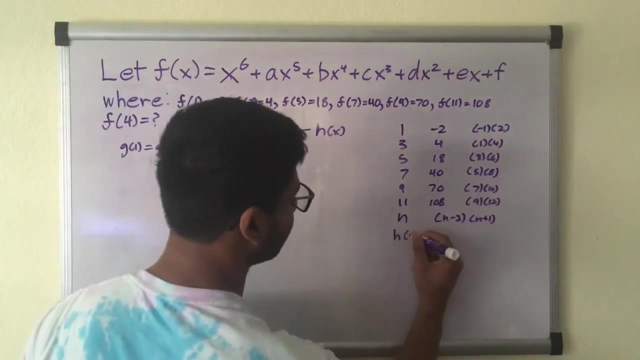 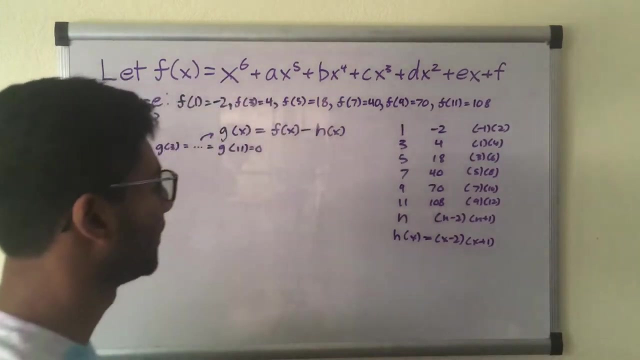 is that when we have an n, our output will be in the form n minus 2 times n plus 1.. So we have an idea for h of x. Our h of x could be x minus 2 times x plus 1, okay. 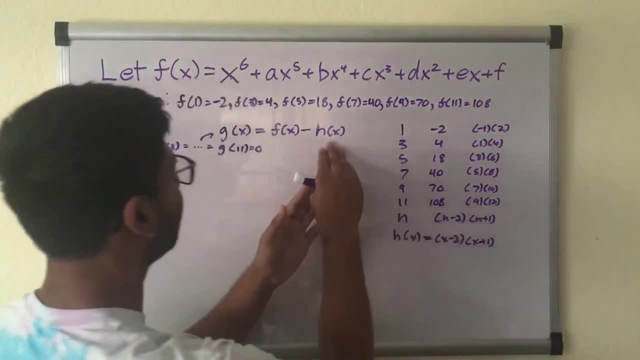 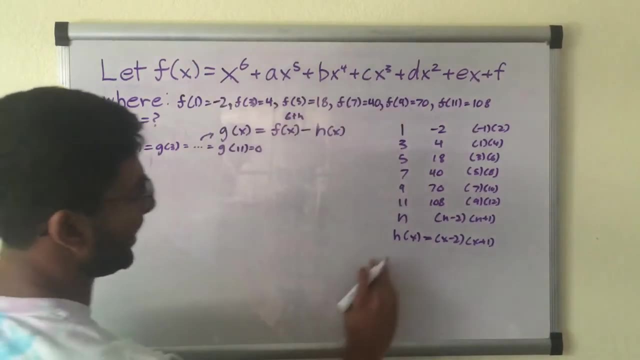 So now what we're going to do is we're going to take this h of x and we're going to put it in, But first let's observe something real quick. f of x is a sixth degree polynomial h of x. well, this will. 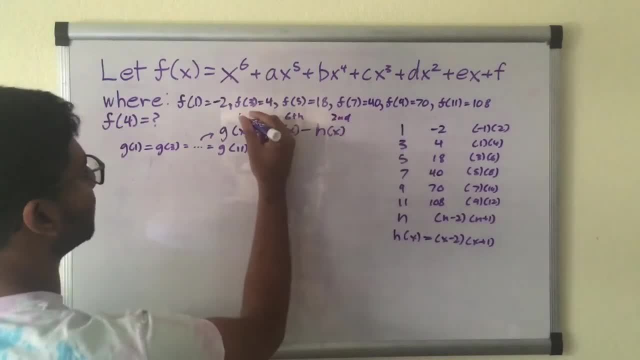 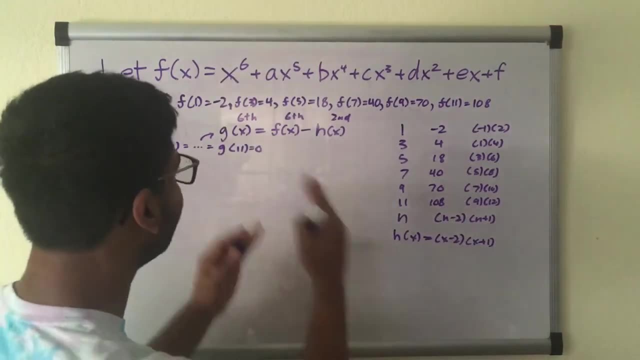 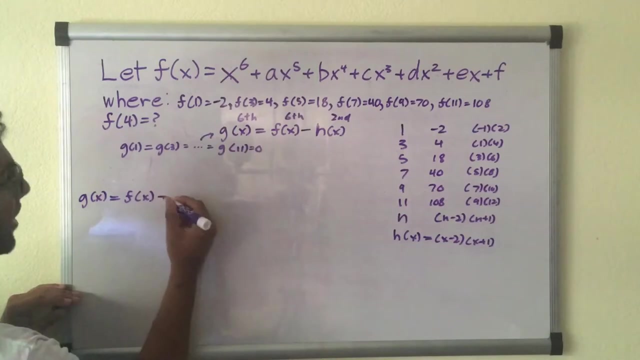 be a second degree polynomial. So this confirms that g of x will be a sixth degree polynomial and these will be the only roots of g of x. With that in mind, let's go ahead. We will have: g of x is equal to f of x minus x minus 2. 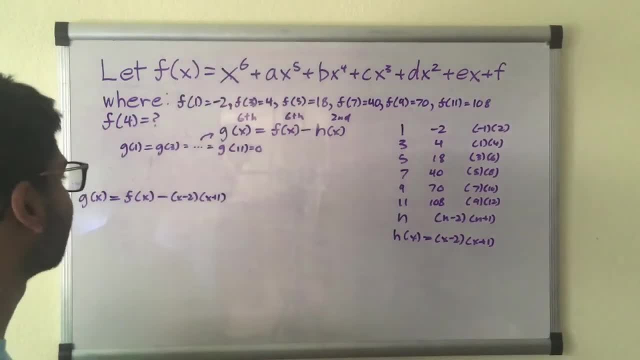 times x plus 1.. Now notice something: Now that we have subtracted this x minus 2 times x plus 1, this is technically equivalent to a factored form, because if we plug the roots in, we'll get 0.. 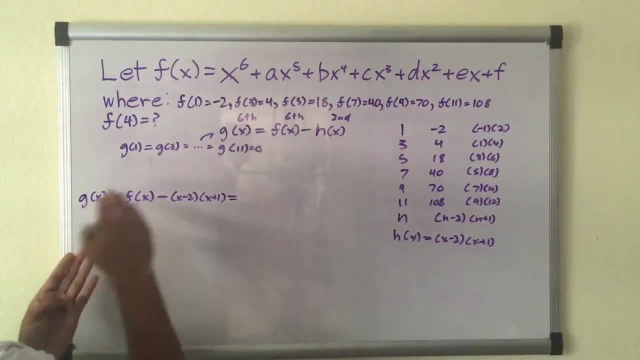 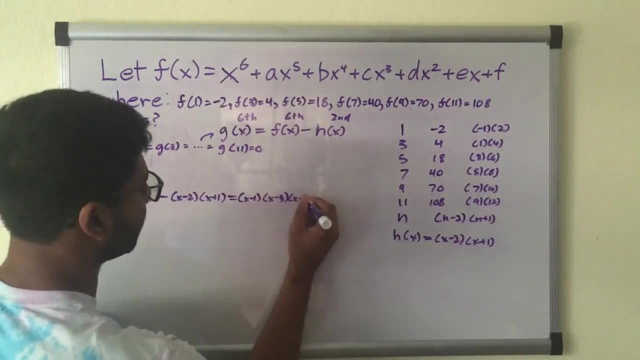 Knowing that we can set this equal to the factored form of g of x, which would be these roots. So that's x minus 1,, x minus 3,, x minus 5,, x minus 7,, x minus 9,, all the way to x minus 11..